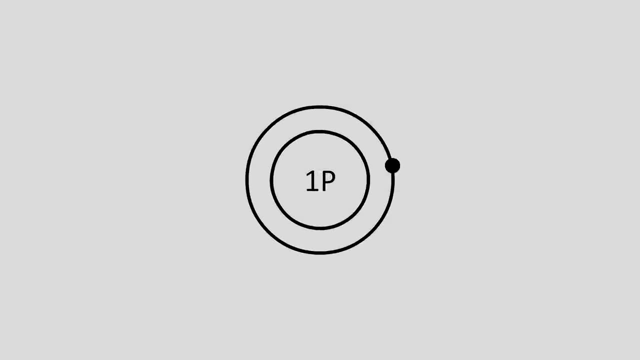 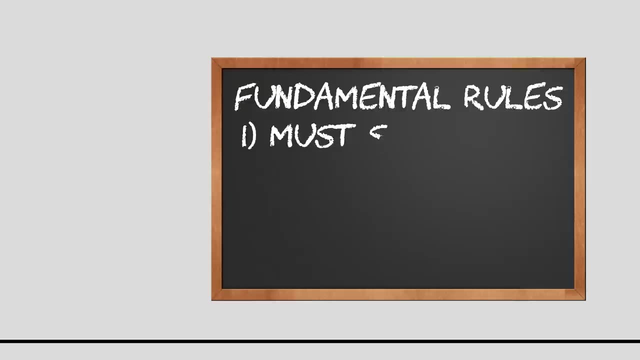 us. This ranges from tiny intermolecular particles to huge things like entire solar systems. Physics argues that there must exist fundamental rules that govern the how of everything around us, and it is the physicist's job to find out what those rules are and apply formulas. 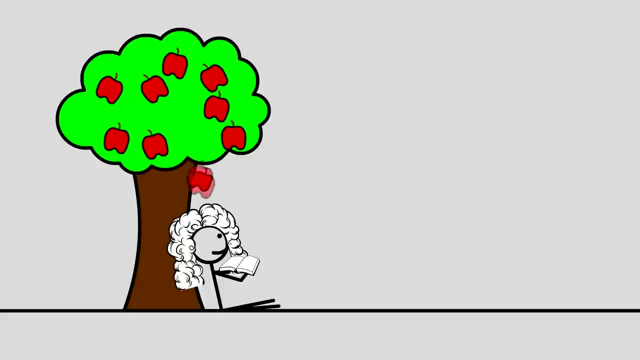 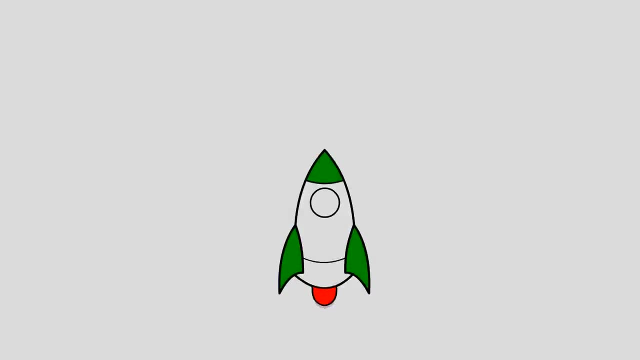 to them. It is really fascinating how much we already know, yet mind-boggling how much we don't. Such simple mechanics such as Newton's famous force-equals-mass-time-acceleration equation can help scientists understand the basic motion. 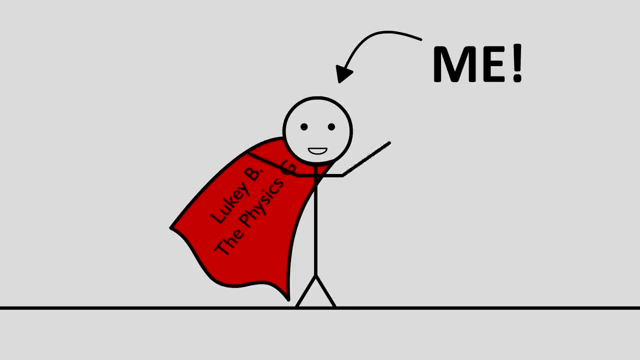 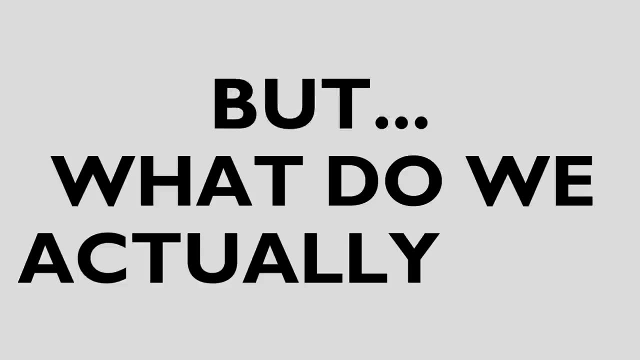 of nearly anything. So I'm here to teach you guys these principles too. That answers what the basic goal of physics is, but doesn't answer what we actually do in physics. Well, in its simplest form, physics is applied mathematics. Now, you've probably 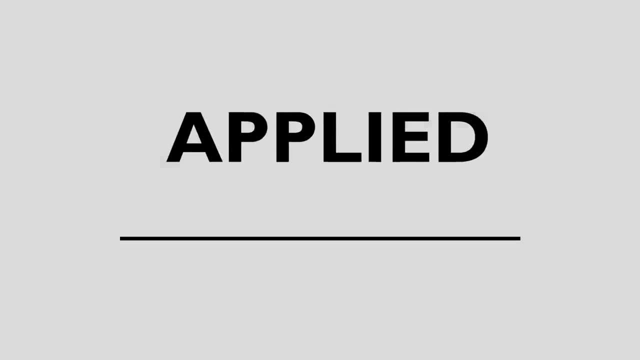 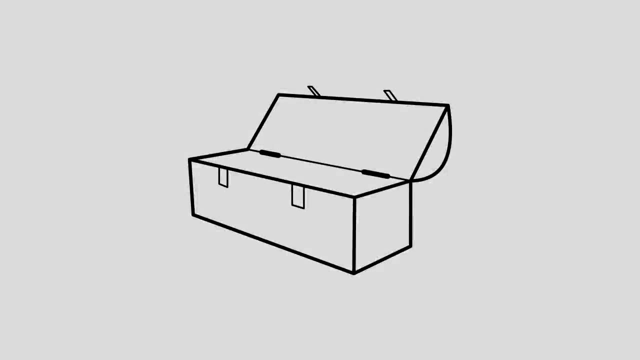 heard the term applied something before, but I'm not sure you really know what that means. To answer that, think about a toolbox. Essentially all of the math you've learned since elementary school are tools that were put into this toolbox. We all start off with an empty toolbox and as we get older and 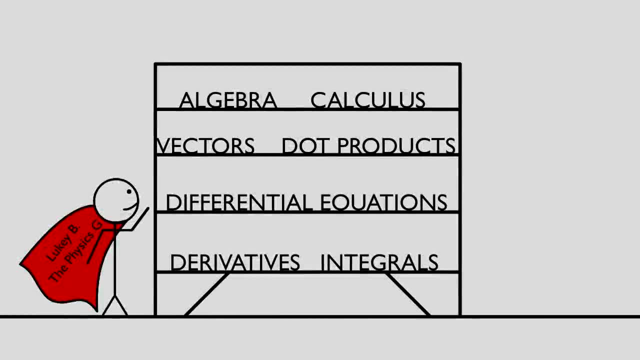 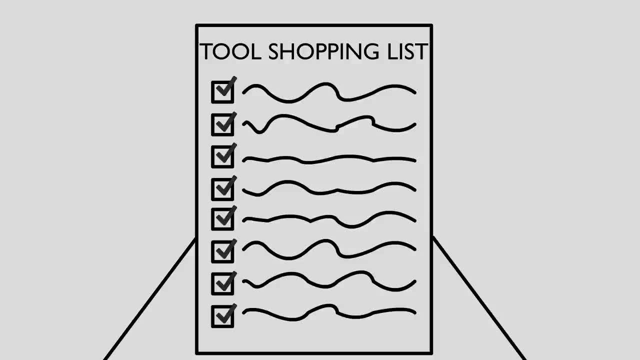 learn more complicated math. we sort of buy and learn how to use new tools. By the time we hit physics, we have a good set of tools that we're very familiar with using, but we never really use them before. See, mathematics is a class that teaches you what the tools. 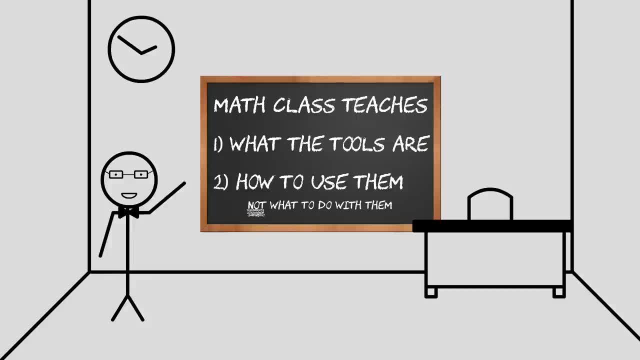 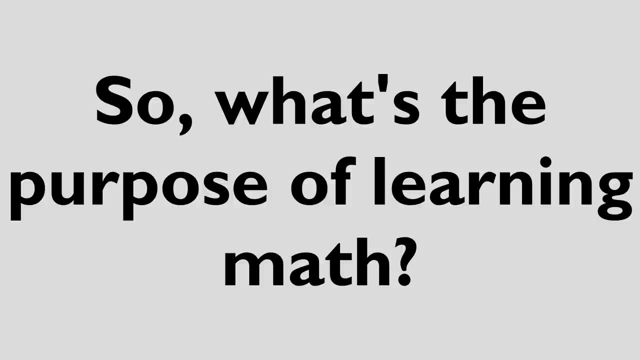 are and refines your ability to use them, but you never truly use them. So what's the purpose of knowing these math concepts? Well, what's the purpose of owning and learning how to use tools To build things? In physics, we take the tools that we learned. 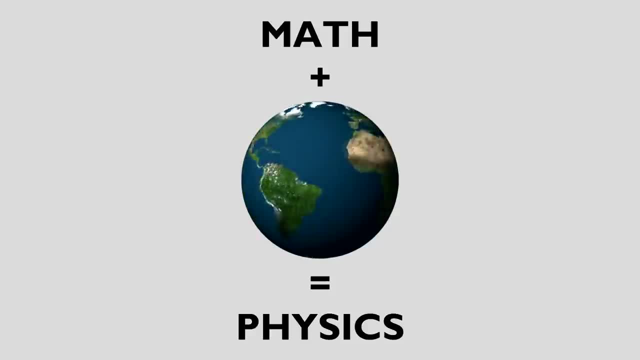 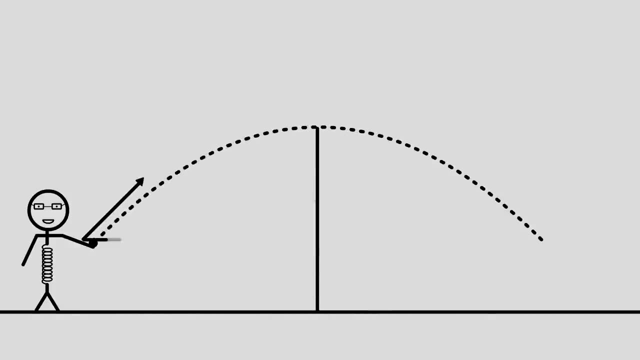 in our math classes and apply them to real-world problems. For example, if we want to find out how high a ball that was thrown upwards will travel, we can use the algebra that we learned nearly two years ago to figure it out. All physics really is is just applying. 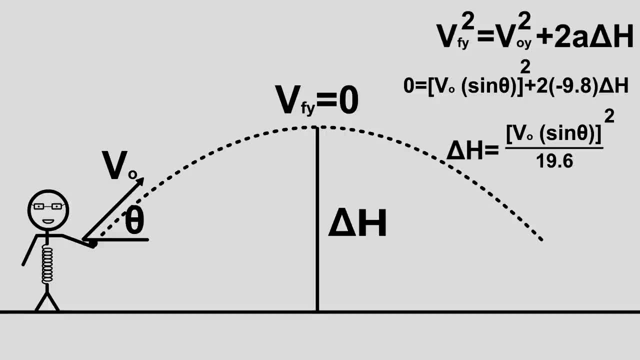 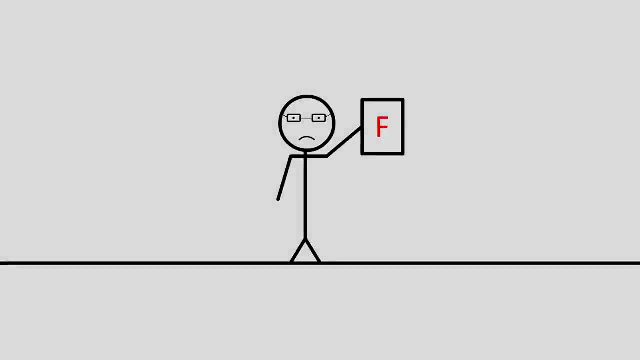 or should I say finally using all of the tools you've accumulated throughout your education to figure out the way the world behaves Now? physics has a bad reputation as being one of the hardest sciences you can take in high school. This can be true, but I believe.